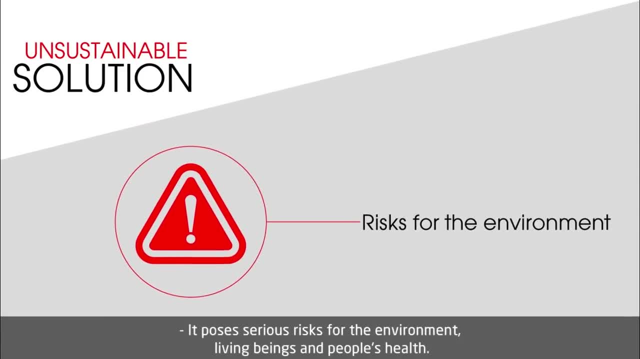 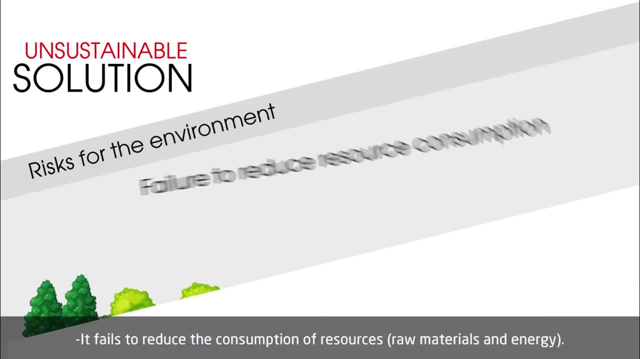 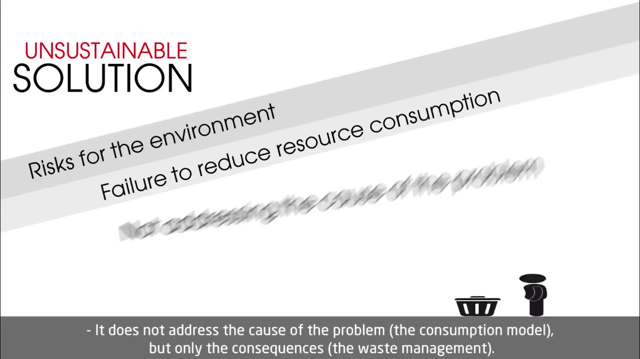 It poses serious risks for the environment, living beings and people's health. It fails to reduce the consumption of resources. It does not address the cause of the problem- the consumption model- but only the consequences: the waste management. Until recently, the production and consumption model was mainly linear. 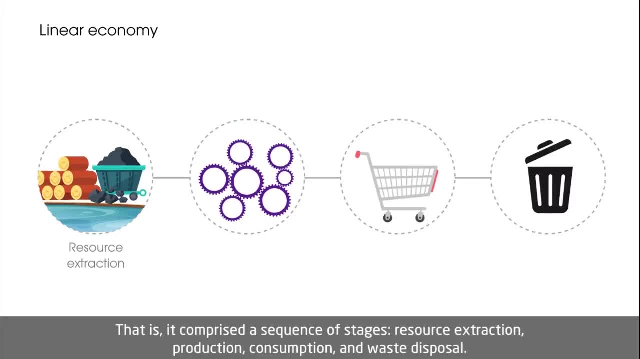 That is, it comprised a sequence of stages: resource extraction, production, consumption and waste disposal. This model in which waste is disposed of is highly polluting as it damages the water in rivers and oceans, lowering the quality of drinking water. 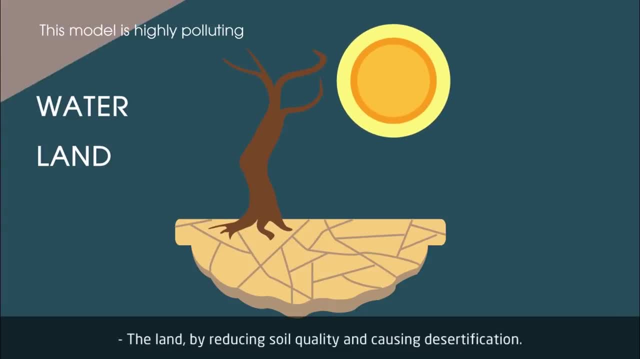 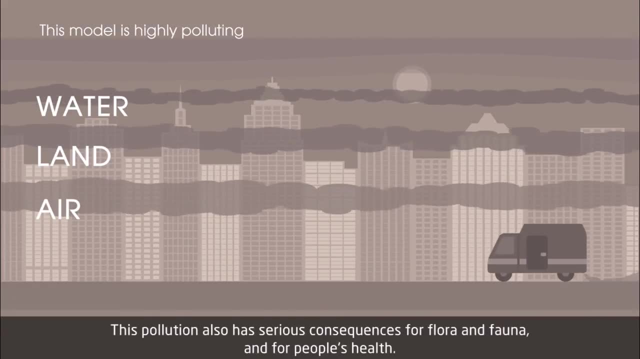 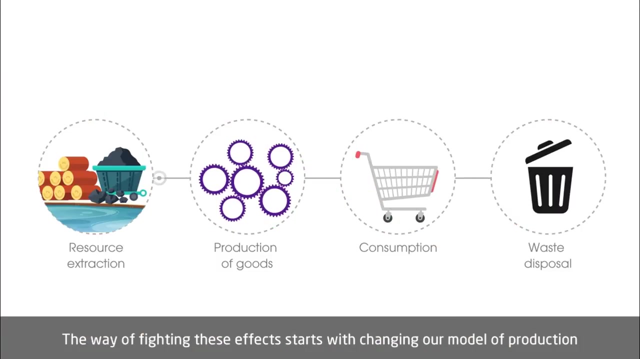 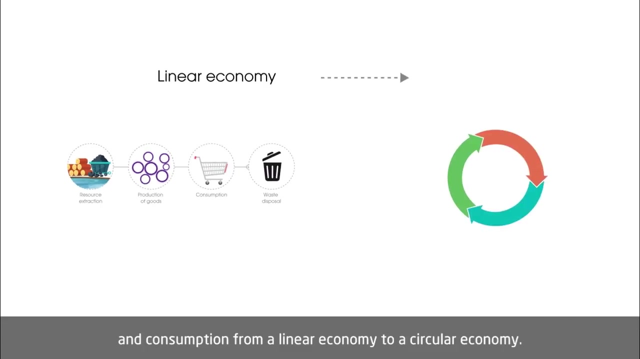 The land by reducing soil quality and causing desertification, The air which becomes polluted, provoking global warming. This pollution also has serious consequences for flora and fauna and for people's health. The way of fighting these effects starts with changing our model of production and consumption from a linear economy to a circular economy. 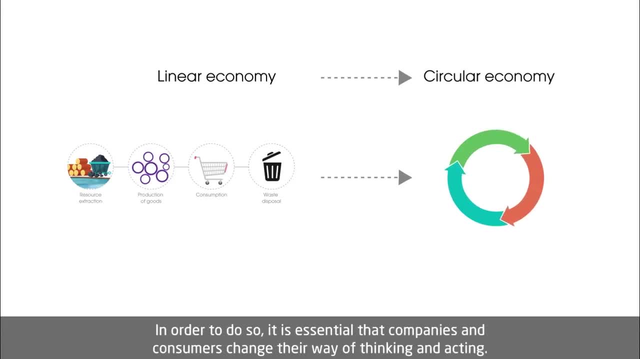 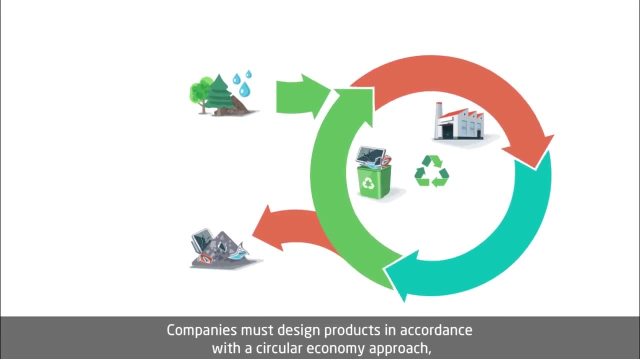 In order to do so, it is essential that companies and consumers change their model of consumption, their way of thinking and acting. companies must design products in accordance with a circular economy approach, using waste as raw materials and reducing the use of resources. but consumers also have a great 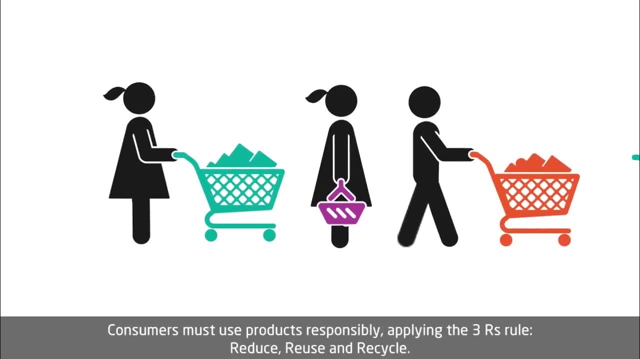 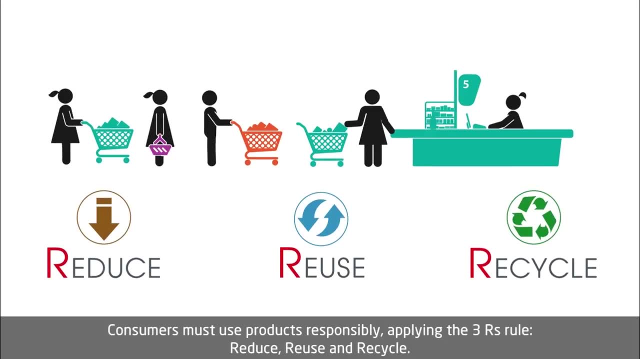 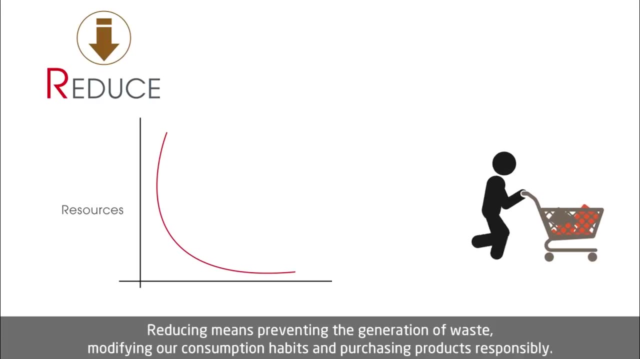 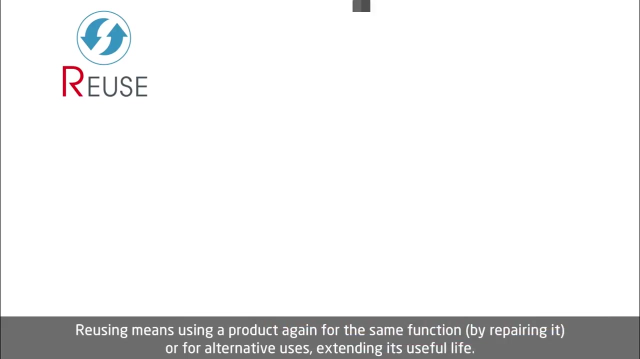 responsibility. consumers must use products responsibly, applying the three hours rule: reduce, reuse and recycle. reducing means preventing the generation of waste, modifying our consumption habits and purchasing products responsibly. reusing means using a product again for the same function, by repairing it, or for alternative uses, extending its useful life and recycling. 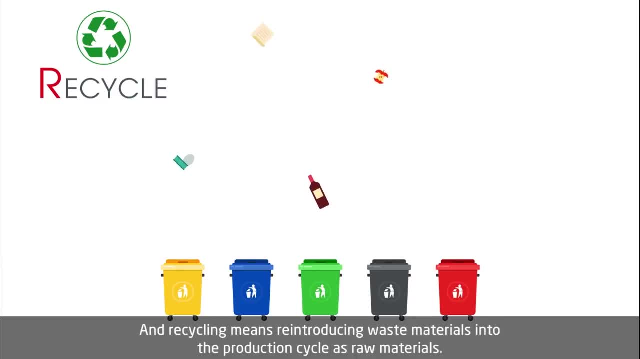 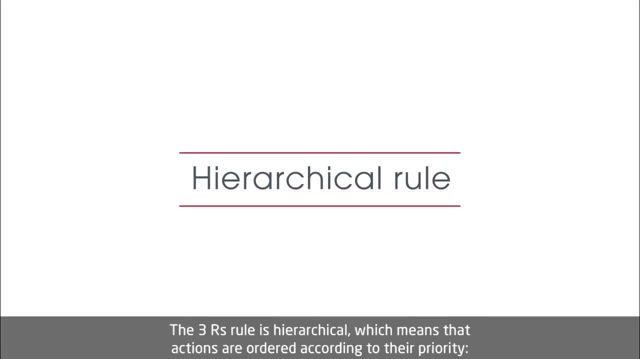 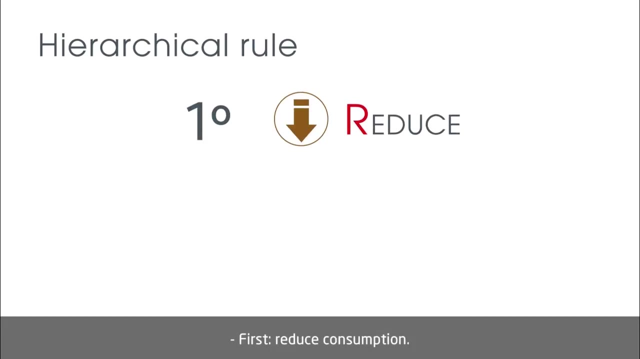 means reintroducing waste materials into the production cycle as raw materials. the three hours rule is hierarchical, which means that actions are ordered according to their purpose and the use of resources and the use of resources priority. first: reduce consumption. second: reuse products. third: recycle only when the first two options are not feasible. how can we do this? here are some.